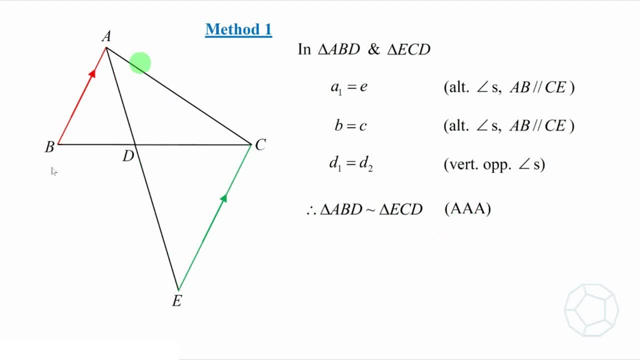 Now we have two pairs of corresponding sides, AB and EC as a pair. DB and DC is another pair. Label the angles as shown in the figure. The ratio of them is equal to E as well. It is possible that are equal. We're going to compare this result with the angle bisector theorem. 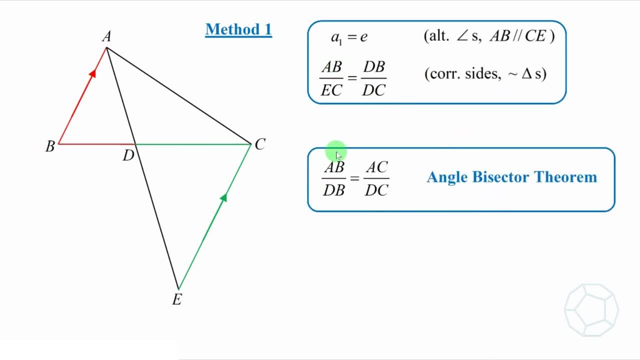 Let's check if all the sides are there. Alright, we have AB, DC and DB. What about the remaining sides, EC and AC? Do they have any relationship? Let's go back to the figure to look at the green triangle ACE We have. A1 is equal to A2. 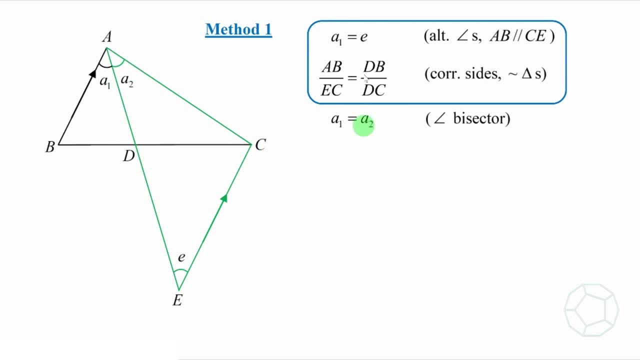 because AD is the angle bisector. Just now we also got: A1 is equal to E because they are the alternate angles of parallel lines. Combining the two results together, we have A2 is equal to E. Therefore EC is equal to AC and the 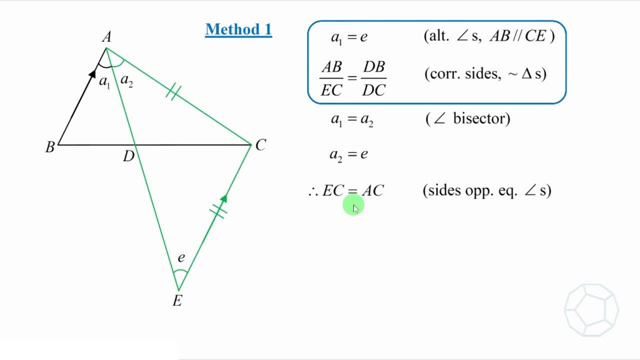 reason is: sides opposite equal angles. Putting this result into the ratio we have, AB over AC is equal to DB over DC. Well, the two red sides, AB and DB, are in the numerator and the two green sides, AC and DC, are in the denominator. Rearrange the terms AC and DB, we complete the proof of angle bisector. 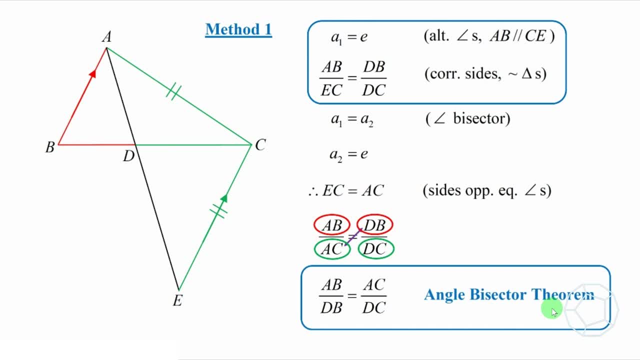 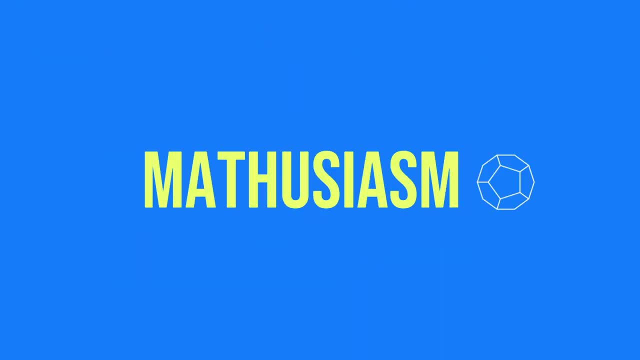 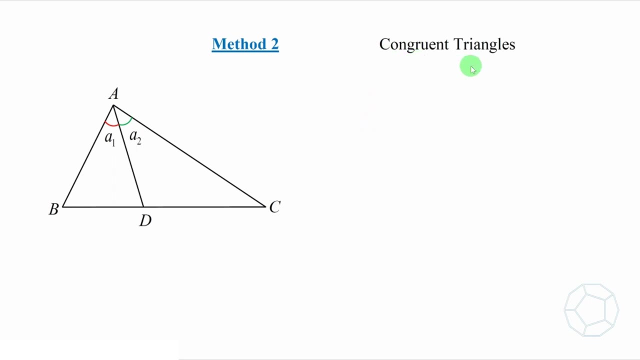 theorem. This method is quite elementary, isn't it? So what about the other two ways to prove this theorem? Apart from similar triangles, we can also make use of congruent triangles To prove that we need both equal sides and angles. Well, do we have that In triangle? 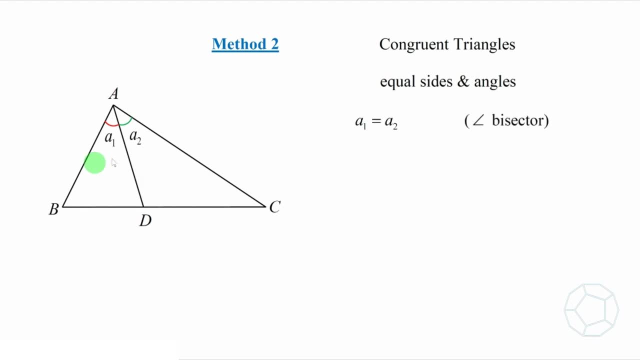 ABD and triangle ACD, A1 and A2 are equal because of angle bisector. Also, AD is the common side. However, the two triangles do not look the same, So we need to draw some lines as well. Let's construct the two heights from the point D. 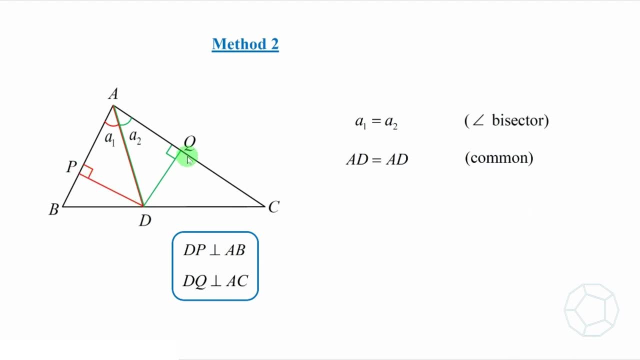 We shall call them DP and DQ. Now we focus on the two smaller triangles, A, dp and triangle ADQ. Then we'll have the two angles X and Y. both are 90 degrees. So we can conclude that triangle ADP and triangle ADQ are. 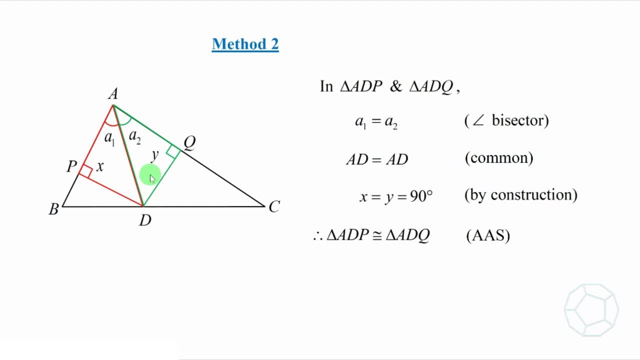 congruent. The reason is aas. as a result, the two heights, DP and DQ, are equal, as they are the corresponding sides of congruent triangles. Well, what else do we know? We can treat them as the heights of the two triangles: the red triangle, ABD, and the green triangle, ACD. In this case, the 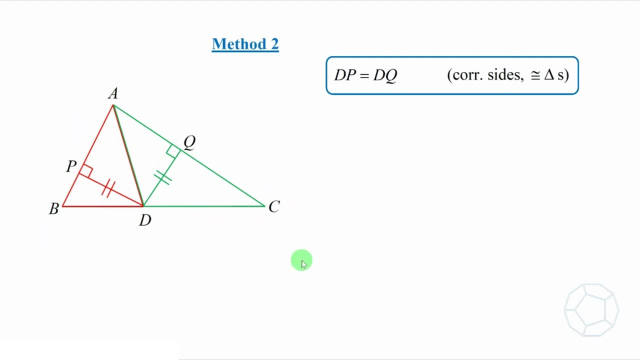 bases are AB and AC. So we can figure out the areas of the two triangles. The area of triangle ABD is equal to 1 over 2 times the base, AB times the height, DP. Likewise we have the area of green triangle, ACD, which is 1 over 2 times the 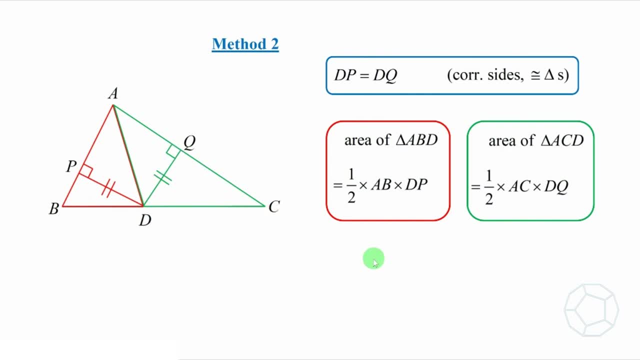 base AC times the height DQ. If we consider the ratio of the two areas, we can do some simplification. Let's take a look at this fraction. Well, 1 over 2 and the equal heights DP and DQ are cancelled, In other words, the ratio of 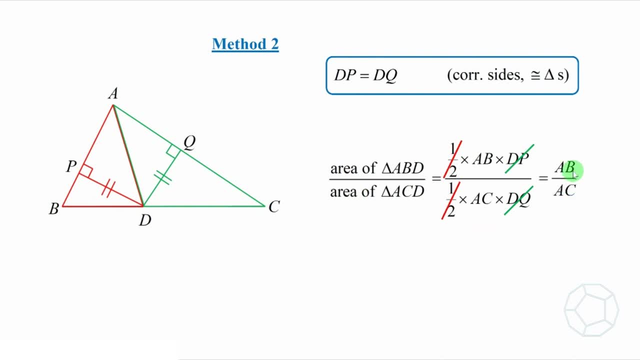 areas is equal to the ratio of the two sides, AB and AC. How is it related to the angle bisector theorem? We have the two numerators AB and AC. Let's take a look at the angle bisector theorem. We have the two numerators AB and AC. 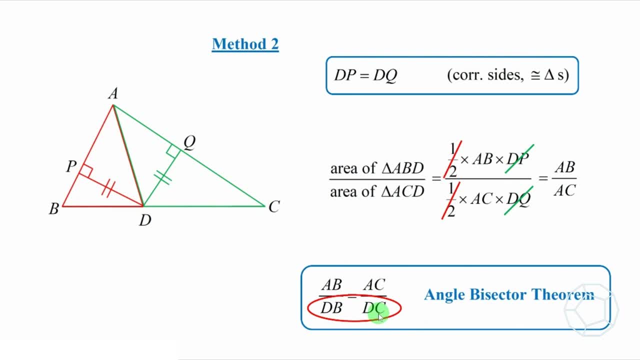 Let's take a look at the angle bisector theorem. We have the two numerators, AB and AC. Let's focus on the two denominators. DB and DC Refer to the figure. DB and DC are horizontal. Moreover, they're also the bases of the two triangles, So we're 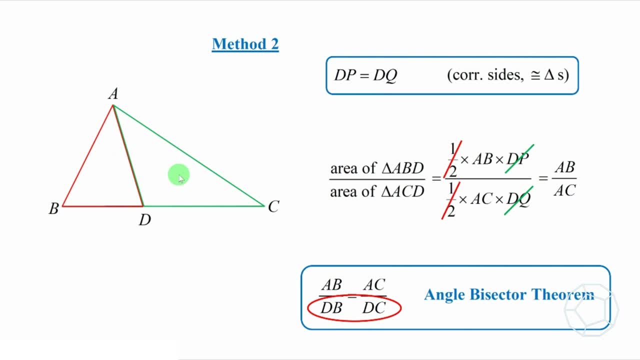 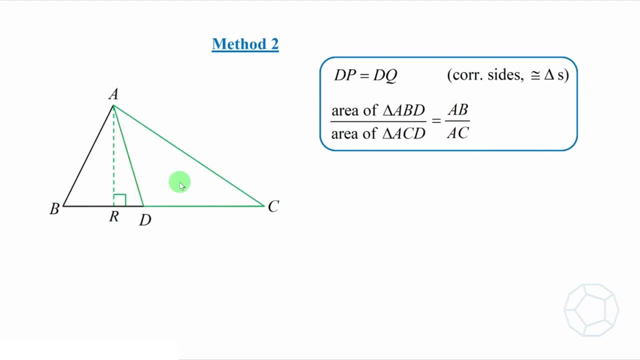 looking at a diagram in another perspective, Now draw the height of the red triangle, ABD, which is AR. Can you see that AR is also the height of the green triangle ACD? Although the two triangles are totally different- one is acute angled triangle and the other is obtuse angled triangle- They share the 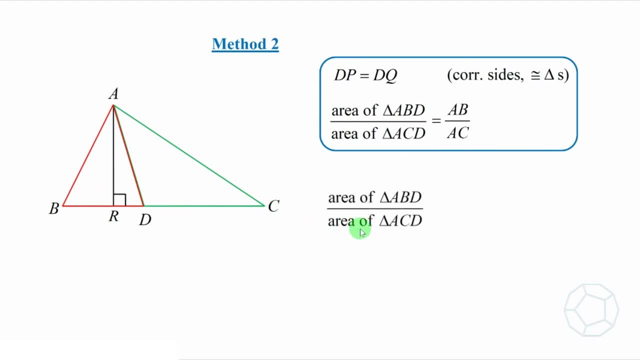 same height. So we can find the ratio of the areas of the two triangles. again. Putting the bases DB and DC and the height AR inside, we get this fraction Again. cancel out 1 over 2 and AR We have the ratio of areas is equal to the. 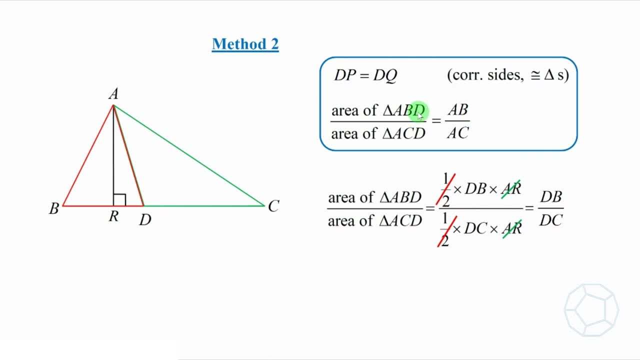 ratio of another pair of bases. Putting two results together, we have AR, So we have AB over AC, is equal to DB over DC. Rearrange the two lengths, AC and DB. We prove the angle bisector theorem again, This time is by the area method. 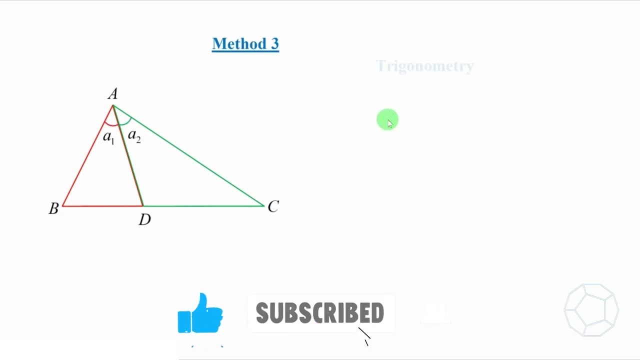 The third method to prove the theorem is to make use of trigonometry. It's also the fastest method. In this case, we don't have to construct any extra lines. Label the two angles as theta and alpha. What can we say further? Let's apply the sine formula in. 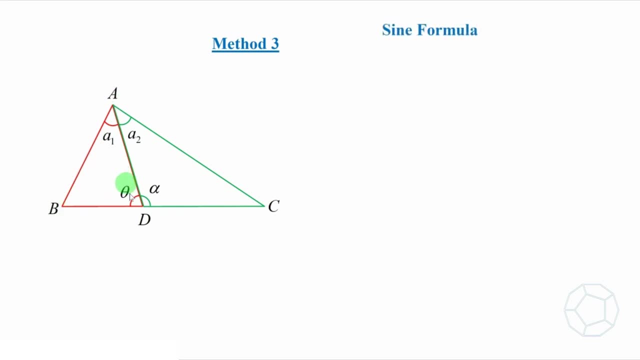 the two triangles, We shall focus on the sine and their opposite angles. In the red triangle, ABD, AB over sine theta is equal to DB over sine a1.. Putting the sine AB and DB to the left and the sine terms to the right, we get this: 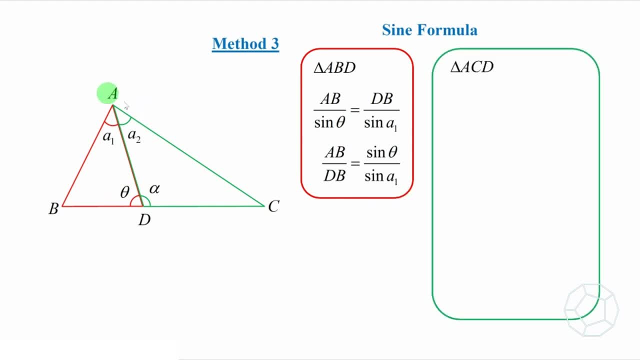 equation- Let's do the same for the green triangle- ACD. AC over sine alpha is equal to DC over sine a2.. Because theta and alpha line on the same straight line. therefore, sum of them is equal to 180 degrees. The reason: 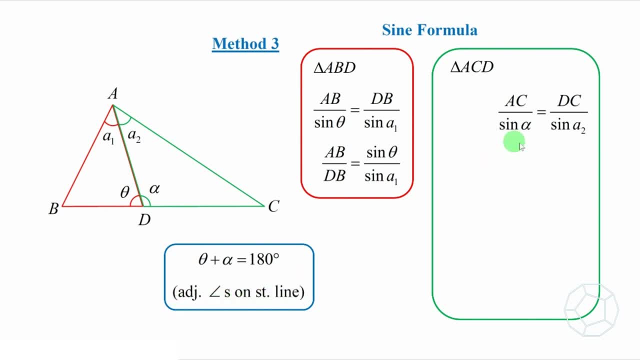 is adjacent angles on the straight line. Therefore, on the left hand side of the equation, alpha is equal to 180 degrees minus theta. Now this sine term can be simplified to sine theta. If we arrange the terms, we get: AC over DC is equal to sine theta over sine A2.. Then 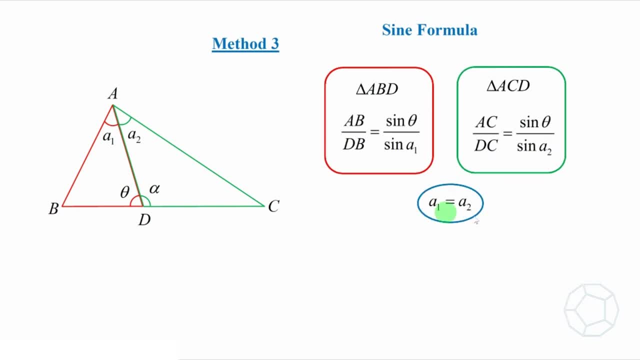 what's next? Let's make use of: A1 equals to A2, again from the angle bisector AD. Therefore, the two fractions are equal. Put them together. the third proof of the theorem is also completed. The ratio of AB and DB is equal to the ratio of AC and DC. We have approached the theorem. 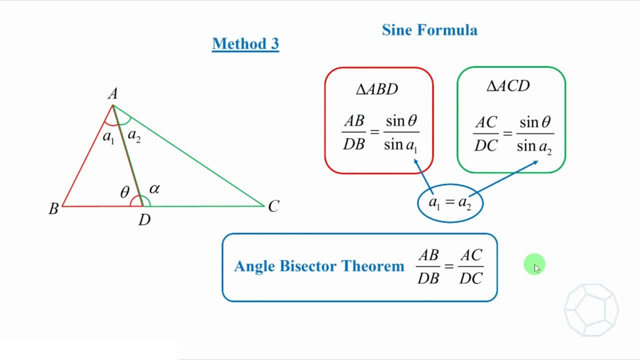 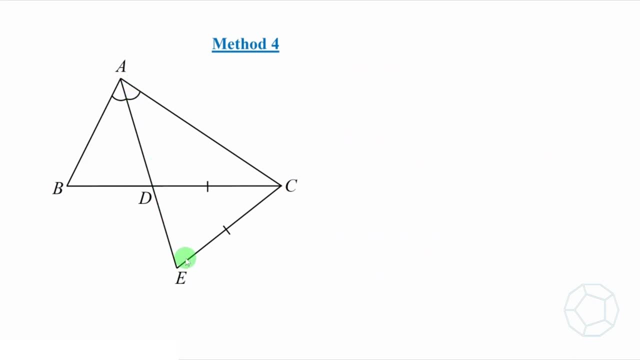 using three different equations. Actually, there's a fourth method to prove that. Let me give you some hints. Refer to this figure: AD is extended to E, so that CD is equal to CE. Then you can prove the theorem using similar triangles as well. We have discussed a lot about the angle bisector theorem, But 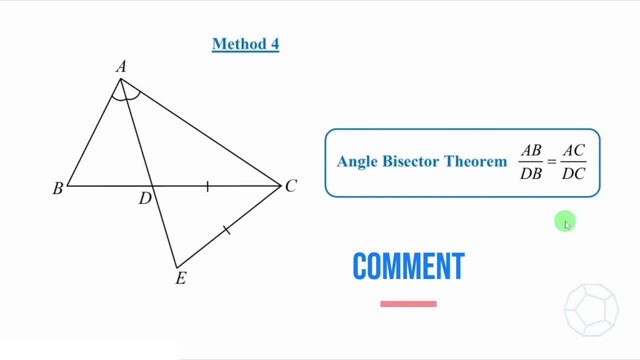 what's so important about that? You may want to check out the next video for an interesting problem. It's solved by this amazing theorem. See you in the next video. Video.